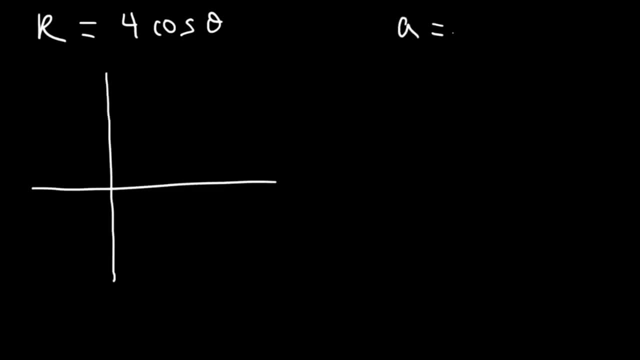 So we're going to have a circle on the right side. Now a is 4, and half of a. well, 4 divided by 2 is 2,, so that's half of a. So what we're going to do is travel 4 units to the right and then up 2 units. 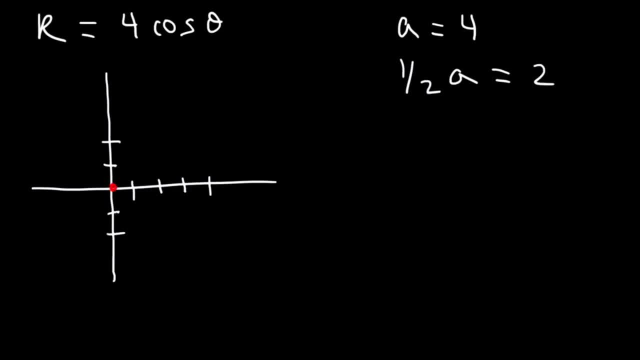 And down 2 units. So the circle is going to start at the origin and it ends at 4 on the x-axis, From the center, which is at 2, we need to go up 2 units and down 2 units. 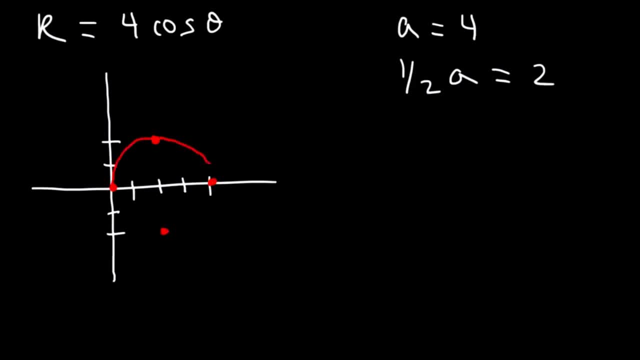 And then simply just connect it. So that's how you can graph: r equals 4 cosine theta. Let's try another one. Try this one. Let's say that r is equal to negative 6. 6 sine theta- I mean not sine, but cosine theta. 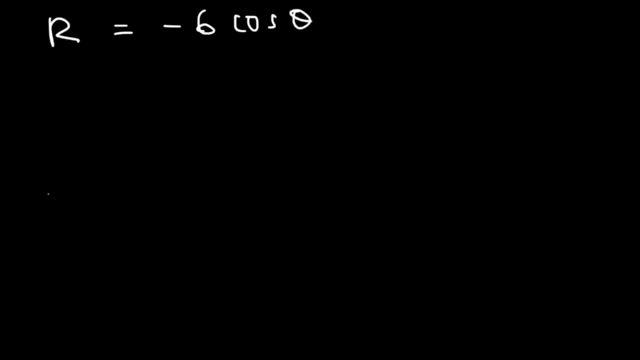 We can get to sine later. Now, because a is negative, the circle is going to be on the left side, on the x-axis, So let's travel 6 units to the right, Since a is negative 6.. One half of a is negative 3.. 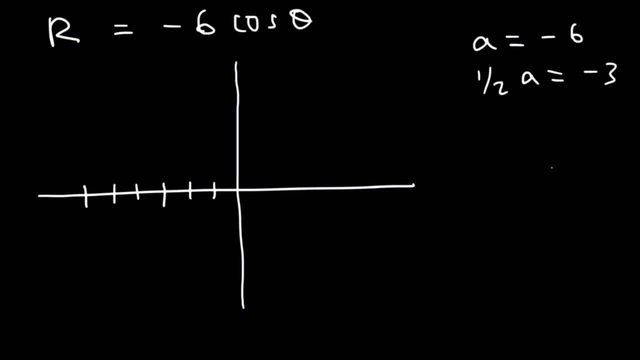 Now, don't worry about the negative sign too much. The negative sign just tells you: if the circle opens to the left Now, the center is going to be at negative 3, which is here. So we need to go up 3 units and down 3 units. 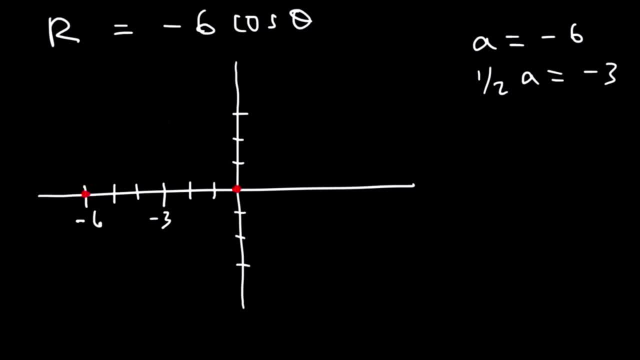 So the graph is going to be at the origin, at negative 6, at negative 3, 3, and at negative 3, negative 3.. And so that's how you can plot the circle. So keep in mind this is equal to. 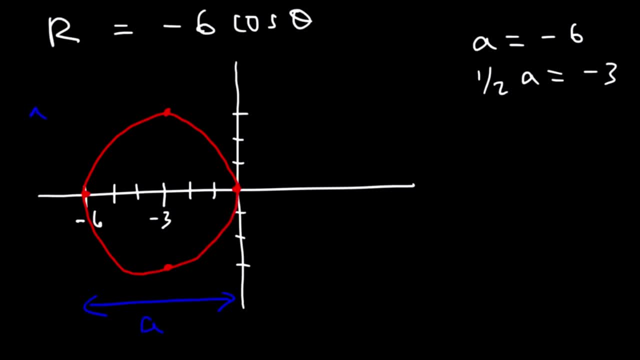 a that distance. and this is also equal to a as well, which means this part is one half of a. So half of a is basically the radius of the circle. So if for some reason, you need to find the area of the circle, you can use this equation: pi r squared. 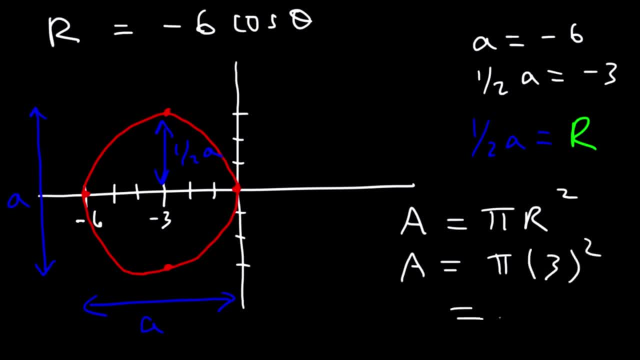 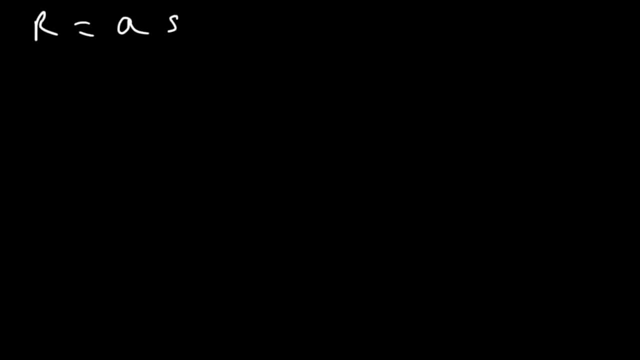 The radius is 3, so it's pi times 3 squared, which is 9 pi. So now the next form we need to know is: r equals a sine. theta Cosine is associated with the x values. So, as you can see, the circle was associated with the x-axis. 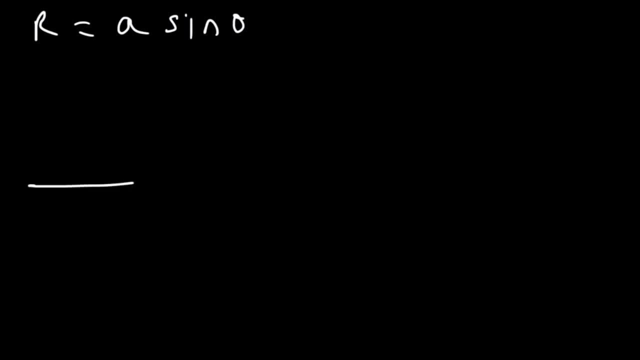 Sine is associated with the y-values, And so the circle is going to be centered on the y-axis. So let's say, if a is positive, then we're going to have a circle that goes above the x-axis centered on the y-axis. 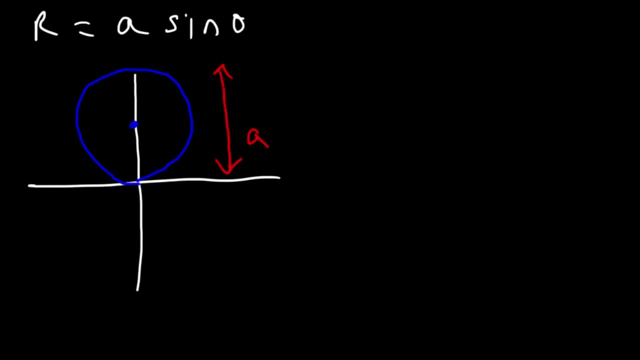 So once again, the diameter will still be equal to a, And this portion, the radius, is half of a. So that's when a is positive or when a is greater than 0. Now, in the other case, if a is negative, 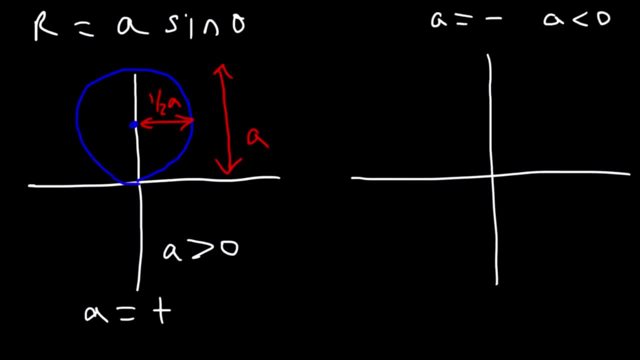 or if a is less than 0, the circle is still going to be centered around the y-axis, but it's going to open in a negative y direction, So it's going to be below the x-axis, And so the radius, as you mentioned before. 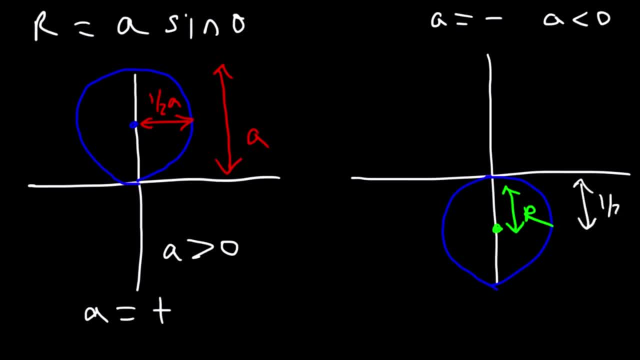 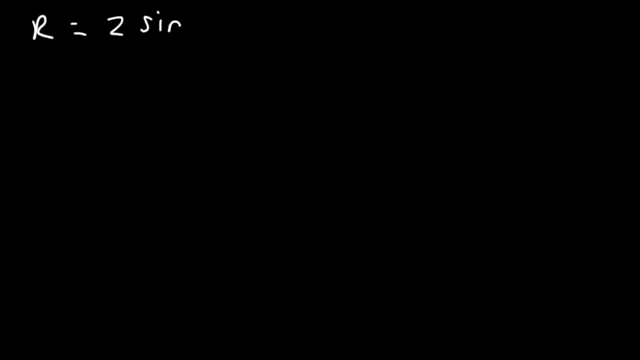 is just one half of a And the diameter is equal to a. So let's try some examples. Let's say: if r is 2 sine theta, Go ahead and graph that. So first we need to travel up two units. a is 2.. 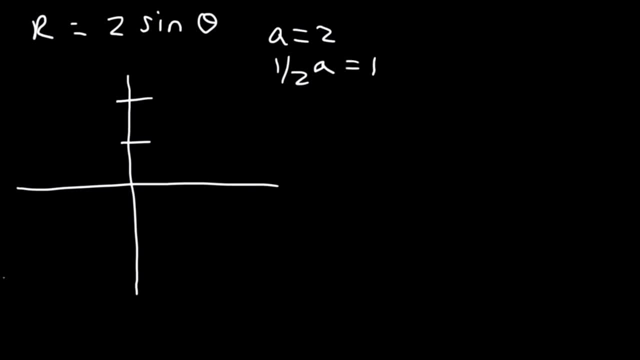 Half of a, which is the radius, is 1.. So we're going to have these two points. Now let's travel one unit to the right and one unit to the left. So the green dot is the center of the circle. 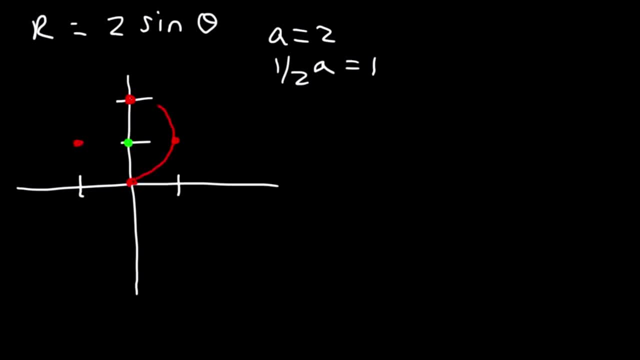 So we're going to travel one unit to the right and one unit to the left from it, And so this is going to be the graph. Try this one. Let's say r is negative 8 sine theta. Go ahead and work on that example. 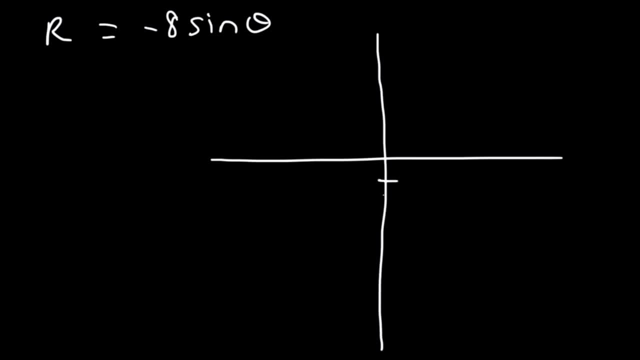 Now the majority of the graph will be below the x-axis, So I'm going to focus on that. So let's travel 8 units down And then half of a or 4 units to the right and 4 units to the left. 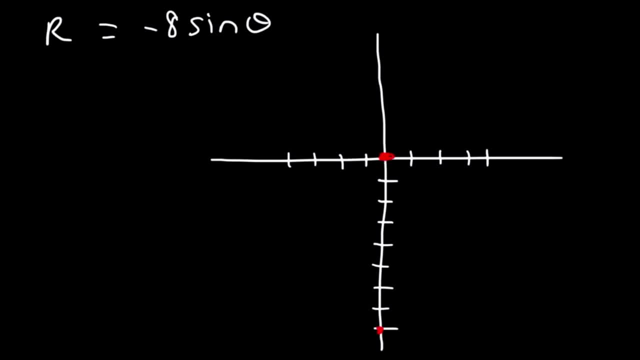 So the point is going to be at the origin and 8 units down. The center is 4 units down. So if a is 8, the radius is one half of a, which is 4.. So we've got to travel 4 units to the right from the center. 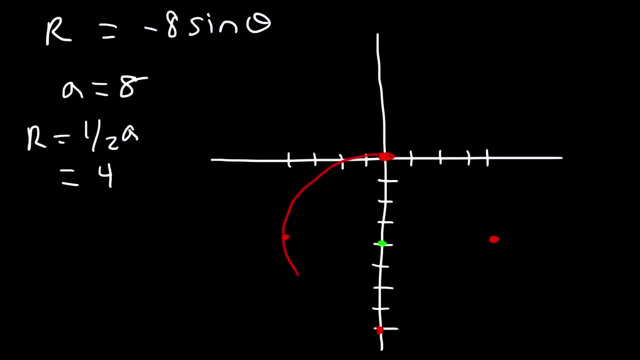 and 4 to the left, And so this is going to be the graph. So now you know how to graph circles when you're given a polar equation. Now the next type of graph that we need to go over is the Lima Song, And the equation is: r is equal to. 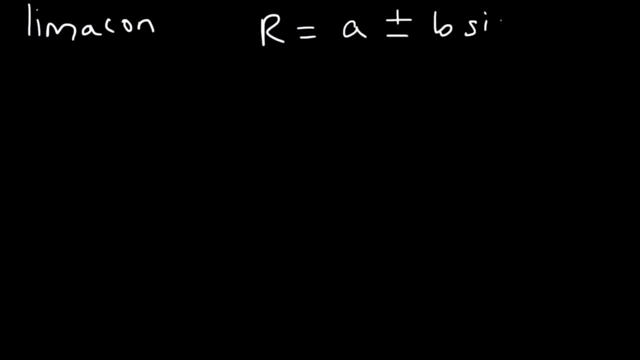 a plus or minus b sine theta. Now, if you have positive sine, it opens towards the positive y-axis, That is, in the upward direction. Negative sine opens in the downward direction, in the negative y direction. You could also have a plus or minus. 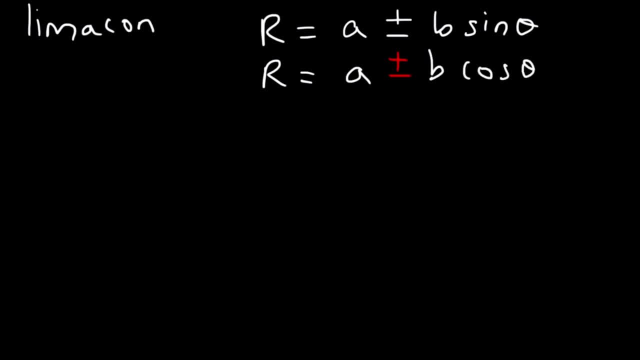 b, cosine, theta. So if cosine is positive, it's going to open towards the right in the positive x-axis direction, And if cosine is negative, it's going to open towards the left. So let's draw the general shape. if it opens towards the right, 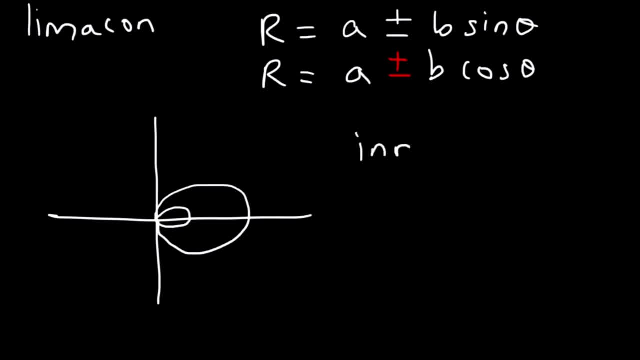 So this is the Lima Song with the inner loop, And you get this particular shape if a divided by b is less than 1.. Now both a and b represent positive numbers. a and b are both greater than 0.. So if you get the graph, 3 minus 4 sine theta. 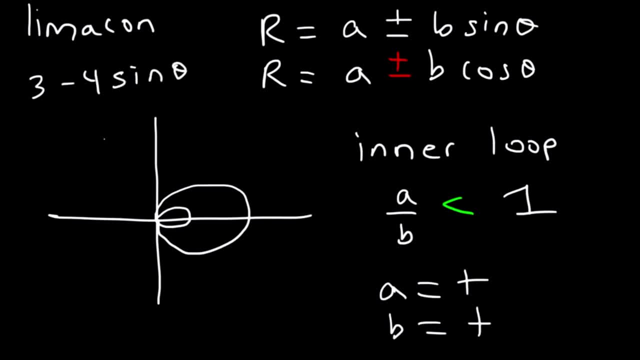 b is not negative, 4, b is positive 4, and a is positive 3.. So let's say, if it was 3 plus 4, cosine theta, both a and b would still be 3 and 4, positive 3 and positive 4.. 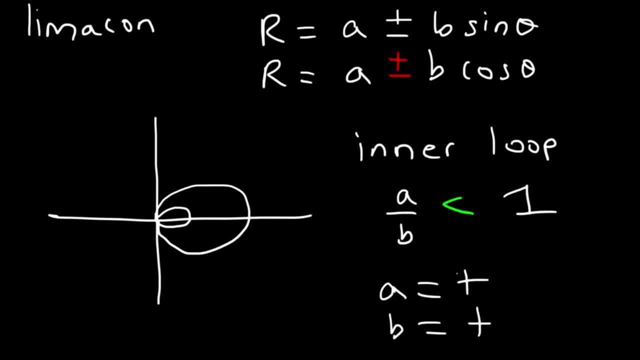 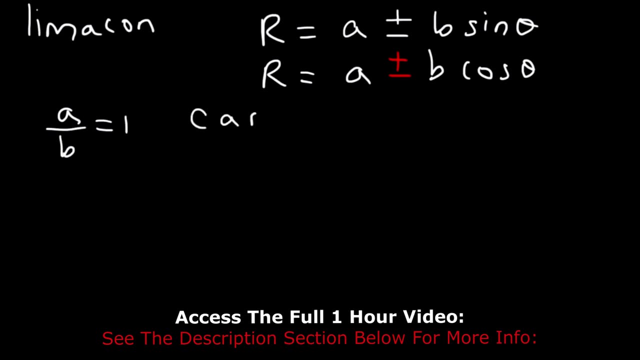 So a and b are not negative. Now the next shape that we have, if a divided by b is equal to 1, is the heart shape, Lima Song, also known as the cardioid, And here's the generic shape for it. So it has like this dimple. 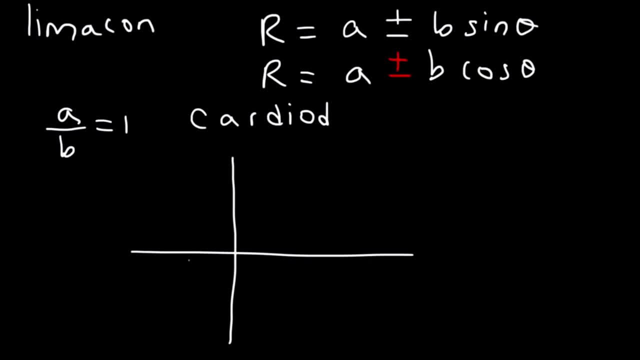 So it looks something like that. Maybe I could draw that better. So that's the cardioid. Now the next one is the dimpled Lima Song with no inner loop. So that occurs if a over b is between 1 and 2.. 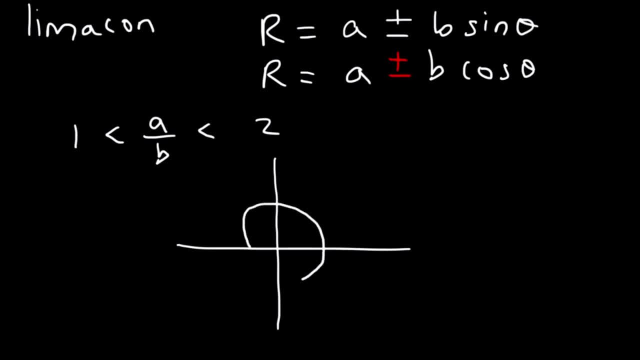 So let's start with the x-axis. It's a small dimple. Sometimes it's hard to notice, So that's the dimpled Lima Song, with no inner loop. The next one you need to know is if a divided by b is equal to or greater than 2.. 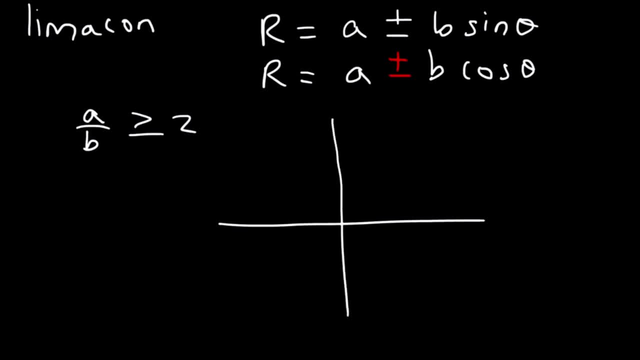 So this Lima Song looks almost like a circle, but it's not. There's no dimple and there's no inner loop. So I'm going to start from the left, I'm going to draw it straight up, And then it looks like this: 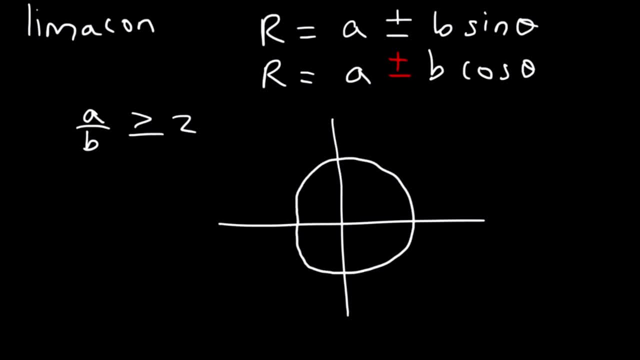 But it's not exactly a circle because, as you can see, the right side looks like bigger than the left, but it almost looks like a circle. So that's the Lima Song, without a dimple or an inner loop. So those are the four shapes you need to be familiar with. 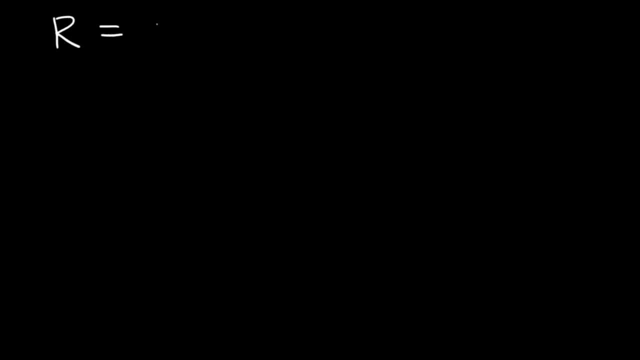 Let's graph this equation. Let's say r is equal to 3 plus 5 cosine. What do you think we need to do here? We know this is a type of Lima Song. It's in the form a plus or minus b cosine theta. 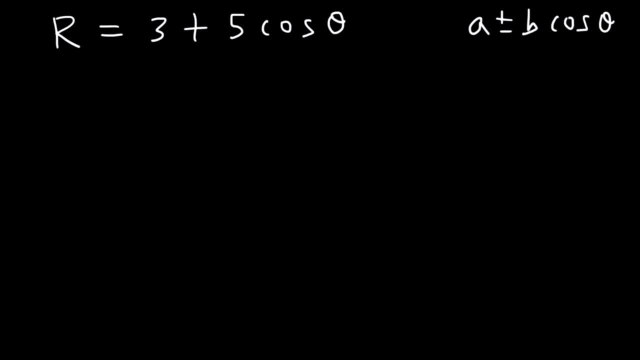 So first we need to identify a and b. a is equal to 3 and b is equal to 5.. Now we need to see if a over b, if it's less than 1, if it's between 1 and 2, if it's equal to 1 or greater than or equal to 2.. 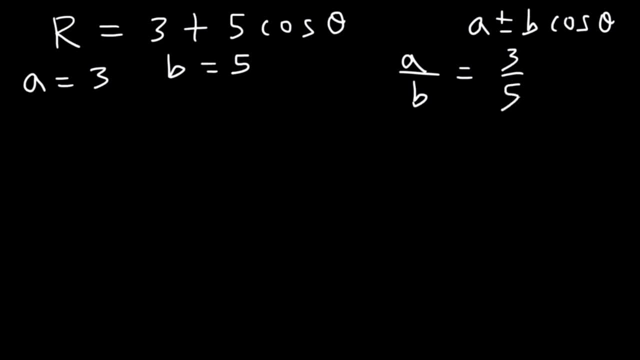 So a over b, that's 3 over 5.. And 3 over 5 as a decimal is 0.6, which is less than 1.. Now, because it's less than 1, we know we have the Lima Song with the inner loop. 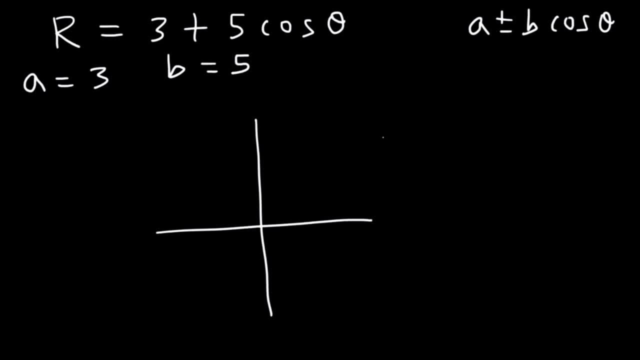 Now there's four types. The first type is: if it's positive cosine, This graph will open towards the right. The next type is if we have negative cosine, And in that case this graph would open towards the left. If it's positive sine. 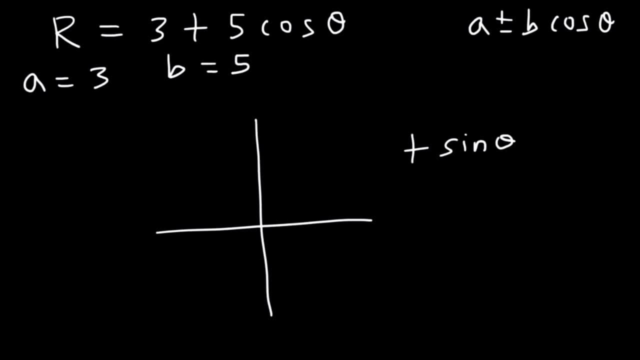 then it's going to open in the positive y direction, And if we have negative sine, it's going to open towards the negative y direction. So it's going to look something like that. So just keep that in mind. That's the first thing that you look for. 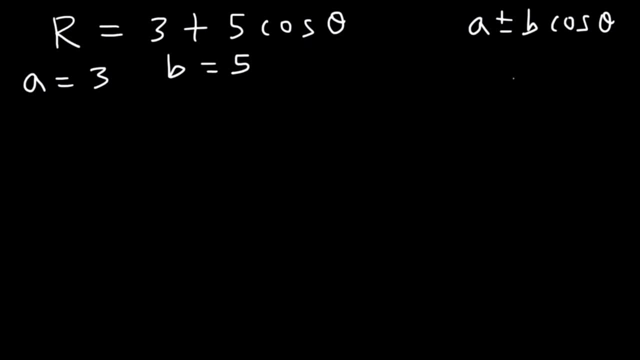 So we have positive cosine, which means it should open towards the right side. Now, when graphing this type of Lima Song, you want to make sure you get four points: Two x intercepts and two y intercepts. So let's draw a rough sketch of this graph. 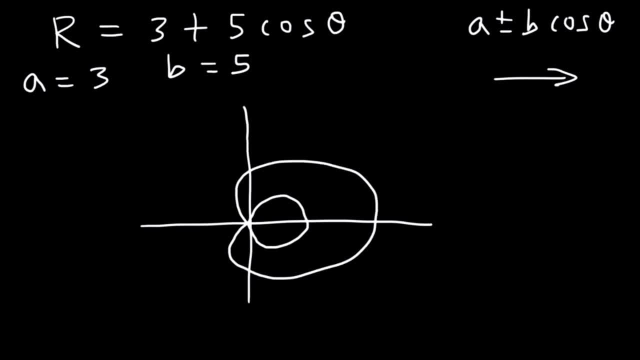 This point is actually positive a, It's a units relative to the center, And this other y intercept is negative a units from the center. The first x intercept, which is associated with the inner loop, it's the difference between a minus b, So it's the absolute value difference. 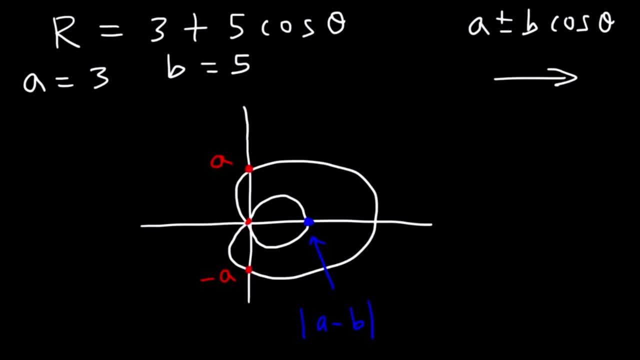 of a minus b, Or you could just say it's b minus a because b is going to be bigger. Now the second intercept is the sum of a and b, And that's all you need to get a good, decent graph If you can plot those four intercepts. 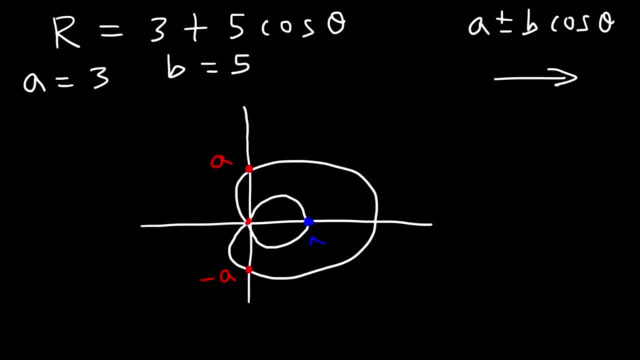 then you should be fine. So let's go ahead and do that. So in this case we can see that a is equal to three. So we need to go up three units and down three units. So those are the y intercepts. Now b minus a. 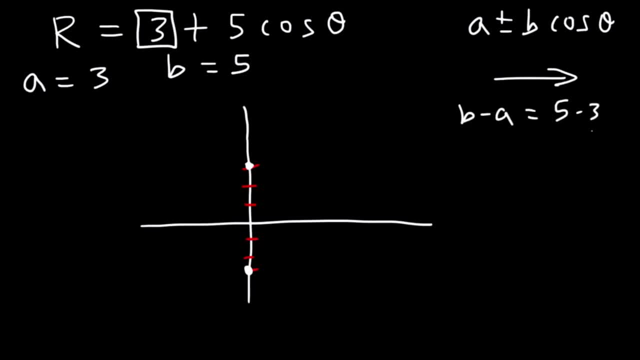 that's going to give us the first intercept, that's five minus three, That's two. So here's the first intercept, And then a plus b. that will give us the second intercept, that's three plus five, which is eight. So that's how you could find the two x intercepts. 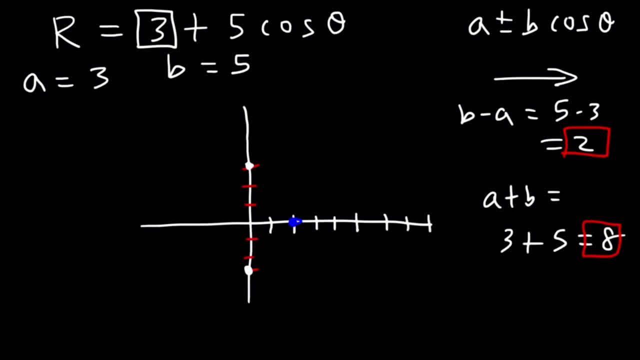 Now let's go ahead and graph it. So first let's start with the inner loop And then let's go towards the first y intercept and then the second x intercept, And then towards the other y intercept. So that's a rough sketch of this graph. 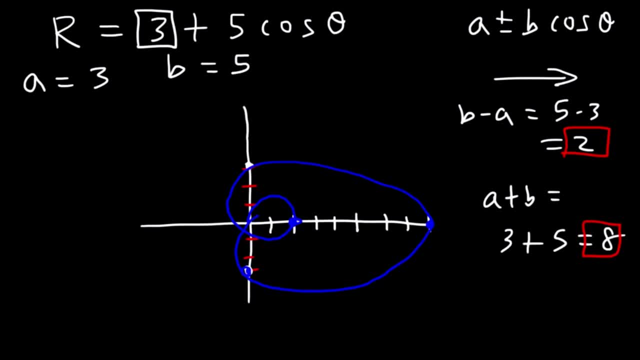 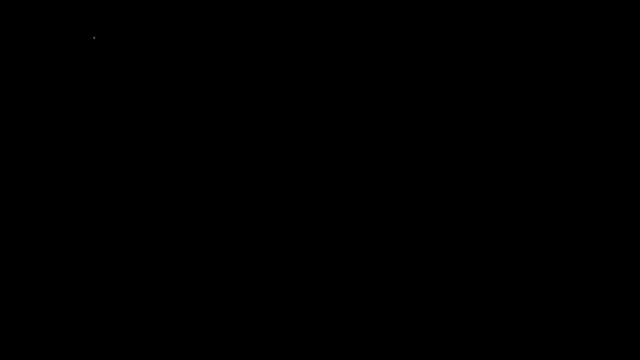 So the points that you need is three and negative three on the y axis and two and eight on the x axis. Let's try another example. So let's say r is equal to two minus five sine theta. So try this one. The first thing I would keep in mind is: 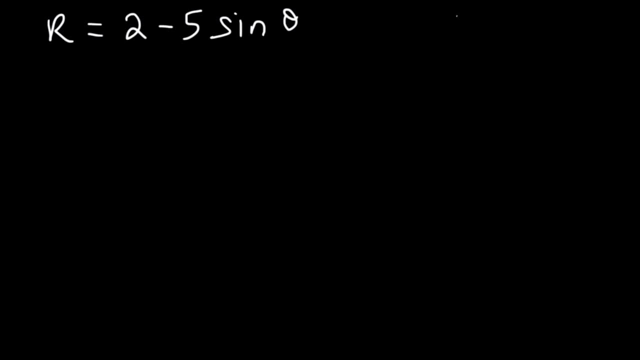 what type of? in what direction will it open? We know that a over b, which is two over five, it's less than one. So this is a lemmasome with an inner loop. But notice that we have a negative sine. 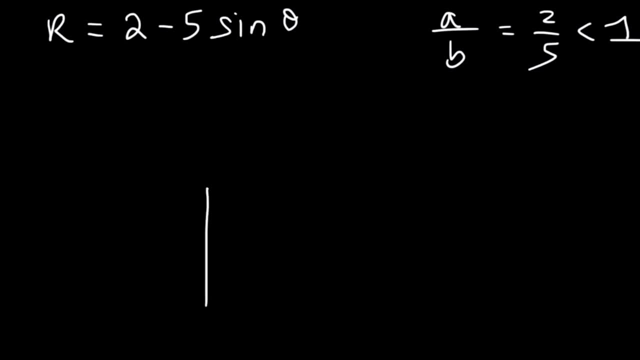 So, therefore, it has to open in a negative y direction. So we can see that a is two- That's going to give us the y intercepts- And b is five. So let's go ahead and graph it Well in this case, because it opens downward. 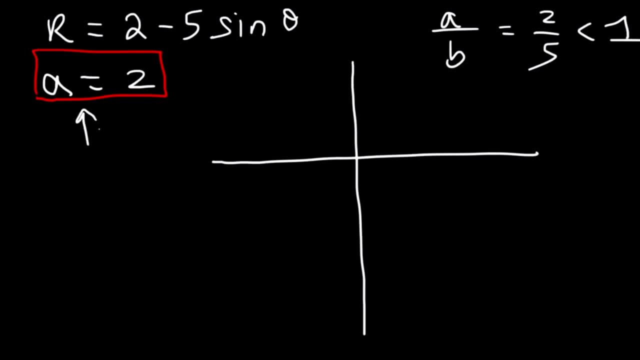 a is actually going to be associated with the x intercepts this time instead of the y intercepts, So it's going to switch roles. So we need to travel two units to the right and two to the left. If we're dealing with cosine, then 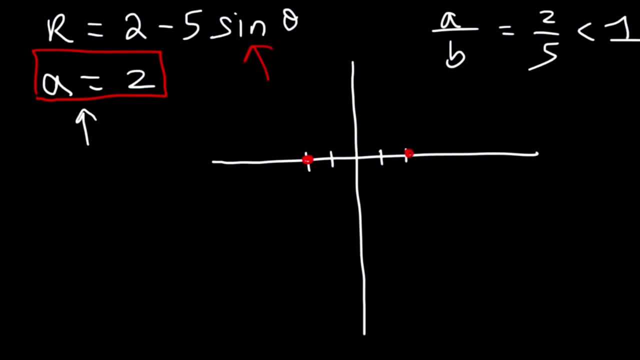 a would be associated with the y intercepts, But because we're dealing with sine, the roles are reversed. Now, a plus b, that's going to be two plus five, that's seven, And b minus a, five minus two is three. 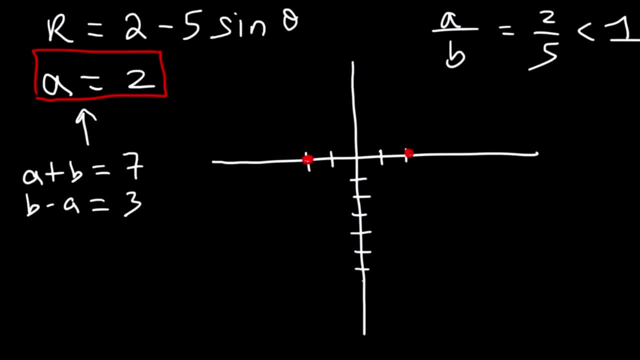 So we're going to travel three units down and also seven units. So we're going to have two y intercepts. So let's start with the inner loop, And then let's let me do that again, And then let's get the x intercept. 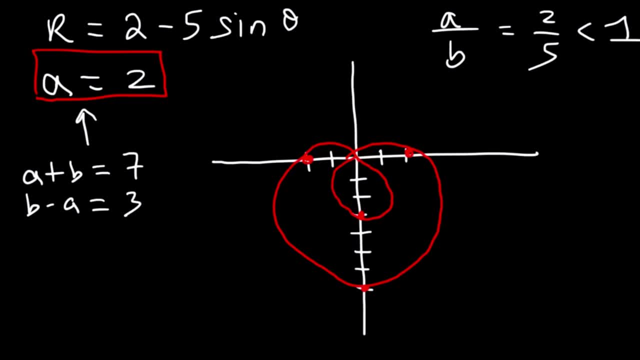 And that's it. So make sure you get these two x intercepts, negative two and two and the y intercepts negative three, negative seven And, as we mentioned before, because we have negative sine, it has to open in a negative y direction. 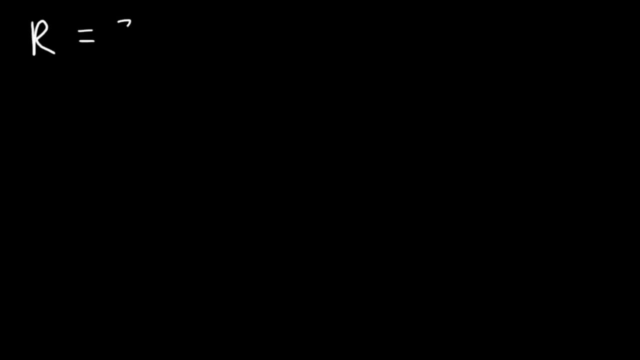 Now let's try this problem. Let's say that r is three minus seven, cosine theta. So go ahead and pause the video and work on that example. So let's find the value of a over b. a is three, b is seven. 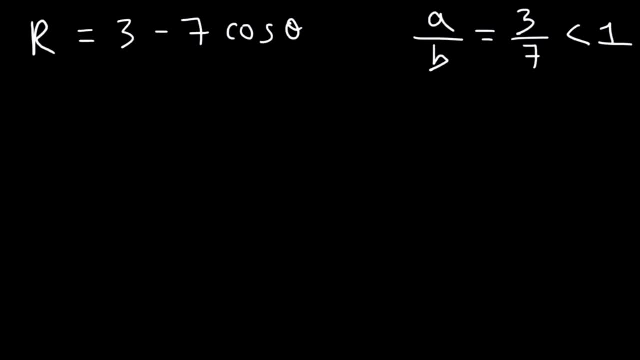 And three over seven is less than one, because seven over seven is one. So what we have is the inner loop limousine. Now we're dealing with negative cosine, which means it's going to open towards the left, So the majority of the graph is going to be on the left side. 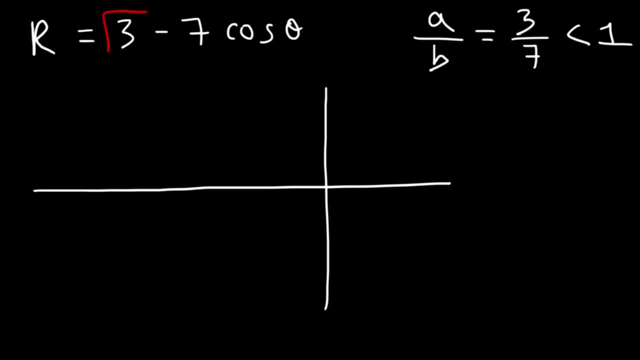 Now a is associated with the y intercepts when dealing with cosine. When dealing with sine, as we saw in the last example, a is associated with the x intercepts. So we're going to travel three units up and three units down to get the y intercepts when dealing with cosine. 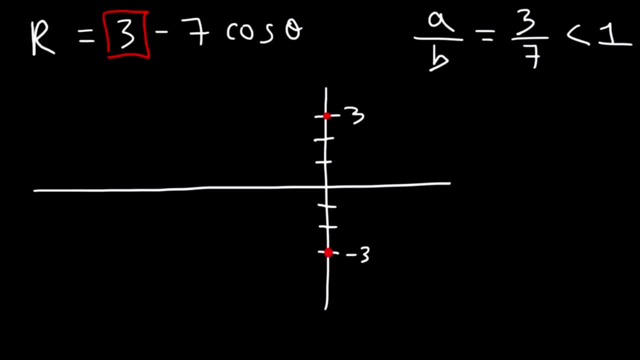 For sine. you need to know that a is associated with the x intercepts. So next we'll find the first x intercept, which is going to be b minus a, or seven minus three, and that's four. And then a plus b, three plus seven is ten. 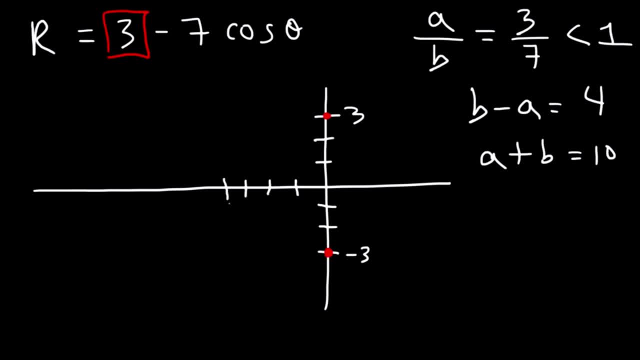 So, because we're going towards the left, we need to travel four units to the left. That's going to give us the first x intercept, And then ten units to the left relative to the origin. So that's the second x intercept. Now let's go ahead and graph it. 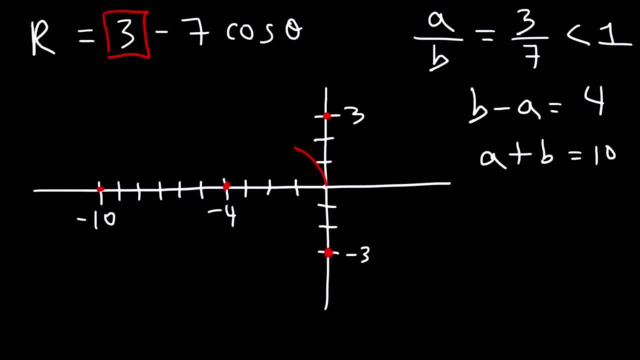 So let's start with the origin and let's draw the first inner loop And then let's focus on the outer loop, And so that's it. That's how you can graph it. My graph is not perfect, but at least that's the general shape. 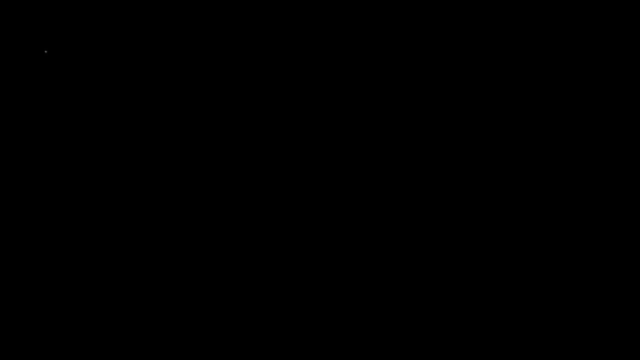 You get the picture. Now let's try this one. Let's say that r is three plus three, cosine theta. What do we need to do here? Well, first we need to determine what type of limousine we have. a and b are the same. 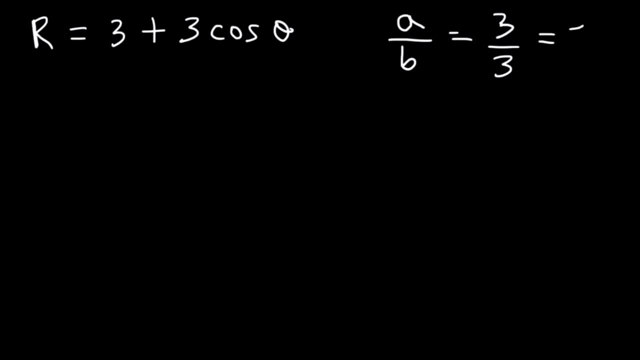 When a and b are the same, a over b is equal to one, And in that situation we have the heart-shaped limousine, also known as the cardioid, And because cosine is positive, it's going to open towards the right. 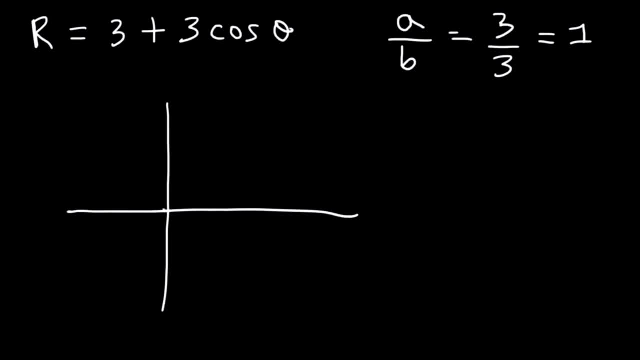 Now I'm just going to draw the general shape of the cardioid, which it looks like this. So there is no inner loop. Now, when dealing with cosine, the x and y-intercepts are going to be a, again a and negative a. 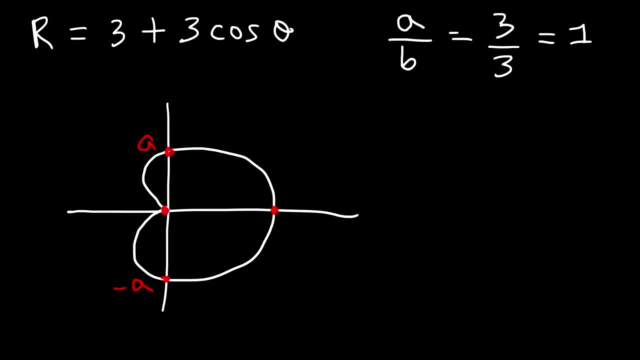 Now, the first x-intercept is just going to be the origin, And so we don't have to do anything. It's just going to start from the origin. Now the second x-intercept is a plus b. We don't have the inner loop. 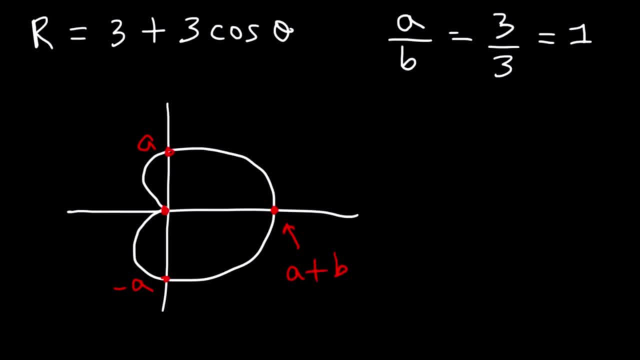 which was a minus b for the inner loop limousine. So we don't have to worry about a minus b or b minus a. So now let's go ahead and graph it. So in this example, a is 3.. So we're going to go up 3 units and down 3 units. 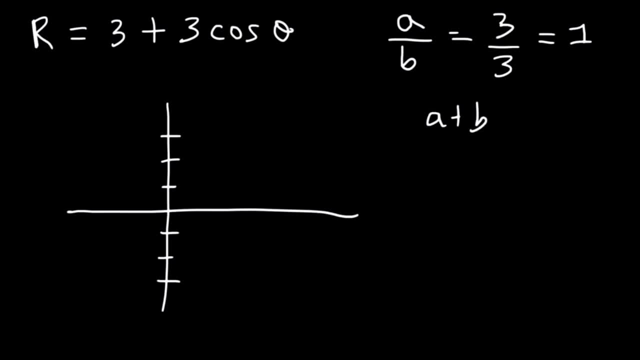 And a plus b, that's 3 plus 3.. So that's equal to 6.. So the x-intercept is going to be 6 comma 0. And the y-intercepts are 0,, 3 and 0, negative 3.. 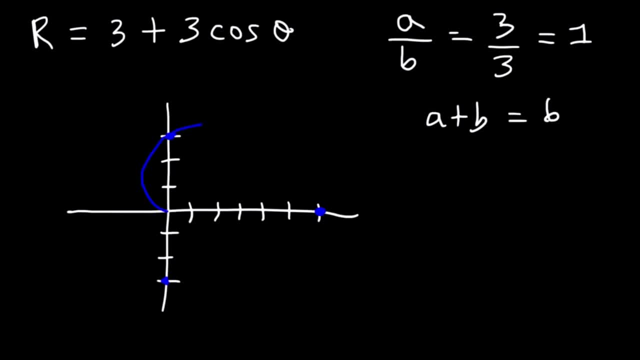 So now that's, We're going to have to graph it like this, And that's it. That's how you can graph the heart-shaped limousine.